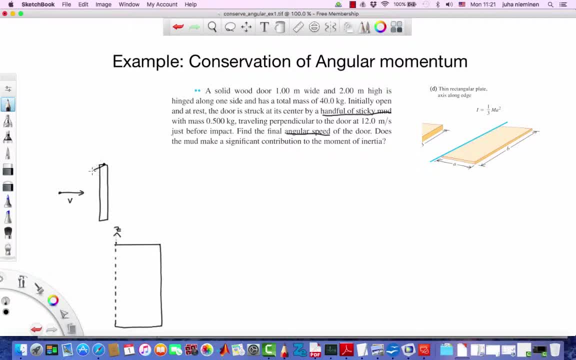 of the door. So it has, or in general case it doesn't matter how far the mud is from the door, And we consider this. So that's the position vector of the mud and the velocity vector, And so we consider it as a particle, So its angular momentum is r, crossed by mv And from. 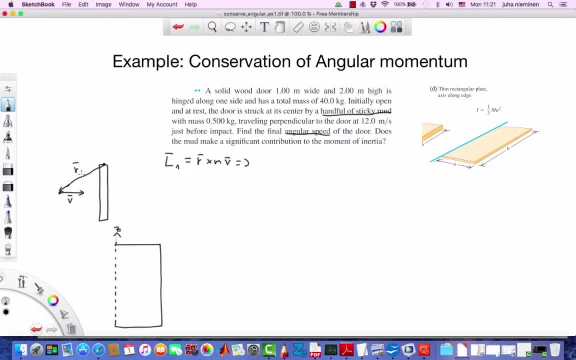 here we are only interested in the magnitude of the angular momentum here. So in that case the cross product becomes m times rv times the sine of phi between those two vectors. So technically the sine phi of phi would be here. But let's say, if this: 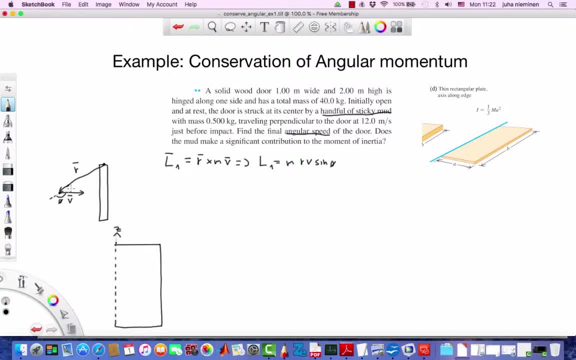 is 30 degrees and that would be 100 degrees. So that would be 100 degrees, So that would be 150.. The sine of that angle is same as the sine of that angle, And what we are really after here is the r sine phi, So this perpendicular distance That is also called the distance. 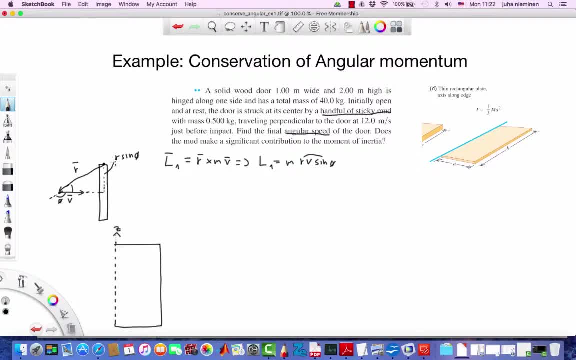 of closest approach, or the lever arm, if you will, And we know that that is just the half of the width of the door. So we get m times rv times, rv times, rv, So l2.. Hence we get m times v times l2 for the. 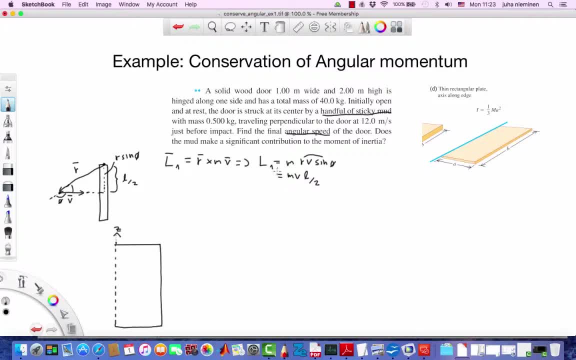 angular momentum of the mud before it impacts the door. What about the angular velocity or angular momentum of the door? So in the overview video I claimed that for object that is symmetric about the axis of rotation, the angular momentum is simply the moment of inertia multiplied by the 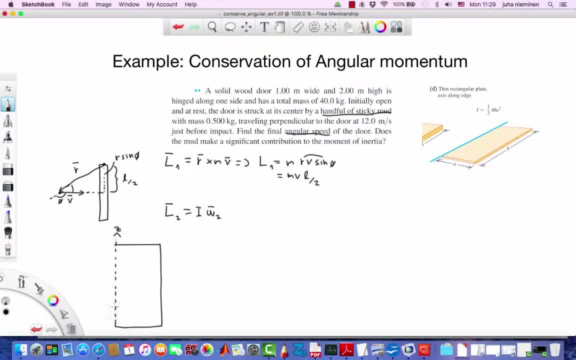 angular velocity. But, as we can see, this story is definitely not symmetric about the z-axis or the axial rotation. So is this relationship true in that case? So let's think about this way. So here we have another axis of symmetry in the other direction. 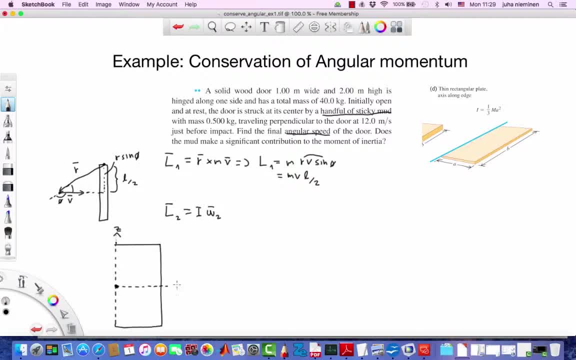 So, and let's have our origin here, This could be x-axis for us, for example. And now let's consider two points that are symmetric about this axis in the door, So like, for example, here. so x means that this point is well. this is, in fact, the velocity vector. 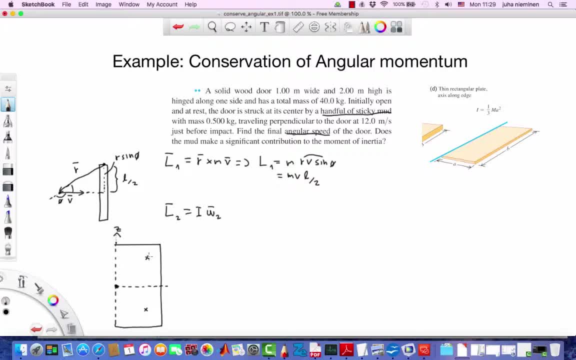 of that point. so this means that it's going into the screen, And so the velocity vector is directed into the screen. So, and then we have the position vector here. Let's call this r2.. And if you take the cross product of, 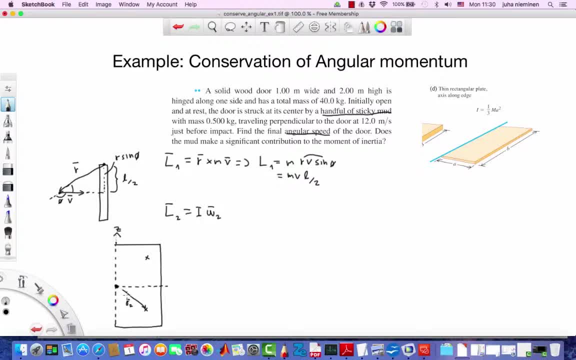 r2 and v2, you can use your right hand rule So you point from the origin into this point, so diagonally down to the right, and you curl your fingers towards the velocity that is into the screen and your thumb will end up pointing in this direction. So that's the angular momentum of that. 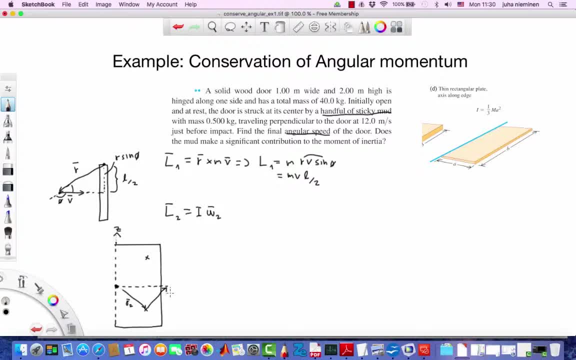 point of mass for that piece of the door. So let's call it. that's a bad subindex. let's call it r3.. So that is l3.. Same thing, the other point that is symmetrically across the x-axis. 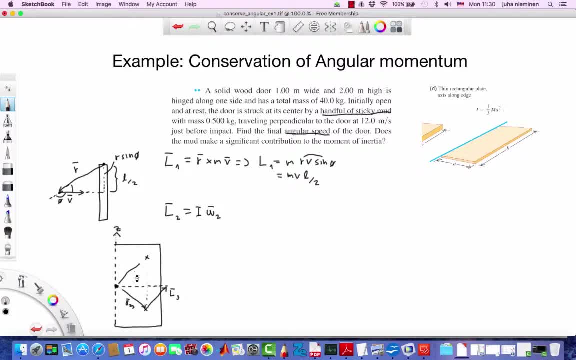 So it has position, vector r4, and its velocity is also into the screen. so point our fingers from the origin towards the x, curl our fingers into the screen because that's what the velocity is. then we say our thumb points to the top left. 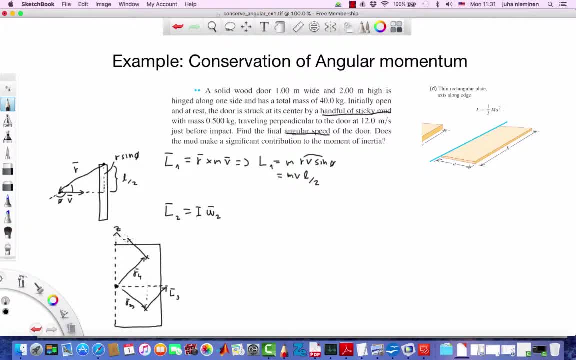 So the angular momentum of that point in the door is in this direction. And now, because of the symmetry, the magnitudes are of course the same: l3 and l4.. They are going at the same velocity and they're equally far from the pivot point or the origin. So 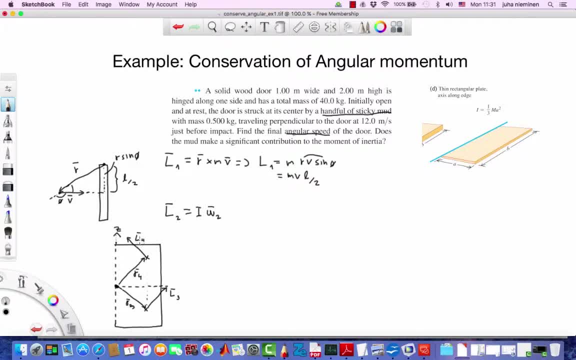 as you can see, the L3 and L4 are off-axis, so they're definitely not pointing in the same direction as the angular velocity vector, which is aligned with the rotation axis, But when we add those two together, L3 and L4,. 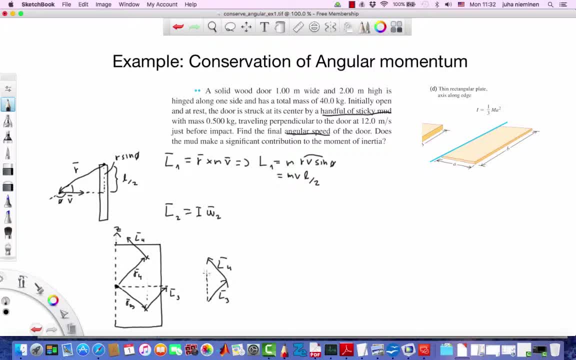 we see that their sum is indeed aligned with the angular velocity. We can repeat this procedure for any two points or pair of points across the symmetry axis, and their vector sum will also add up into a vector that is aligned with the angular velocity. So we can go ahead and use this relationship for the angular momentum And note that. 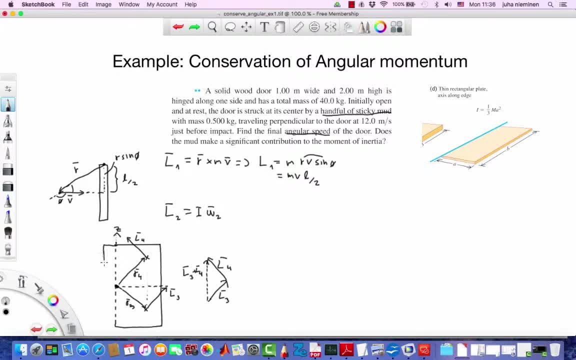 we could have even had the door shaped like this, so the axial rotation would be somewhere within the door and in the same way the point here would cancel the vector sum of these two points. their angular momentum would add up into a purely vertical component. 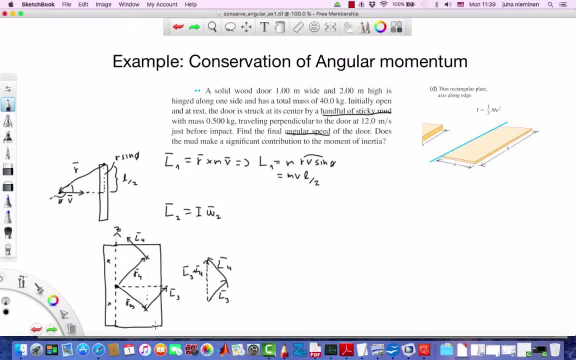 So we are saved by the symmetry. But, for example, if we started chipping pieces away from this door, then this symmetry would break down and this relationship would not hold. But we are good to proceed back into this problem. So what do we need for? 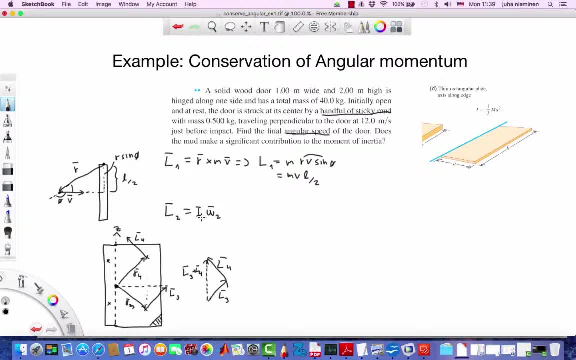 L2?. So we need the moment of inertia after the impact and that's going to be the sum of the angle or moment of inertia of the door plus instead of the mud. so like this. So if we add these two together, so from the door. 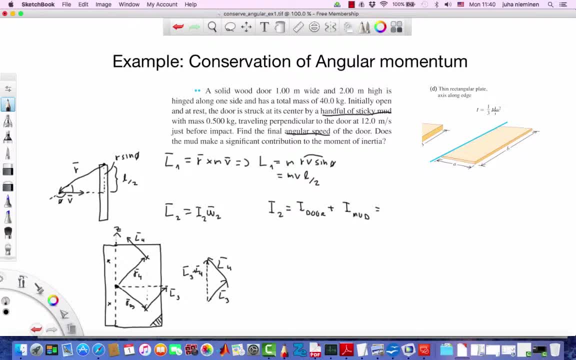 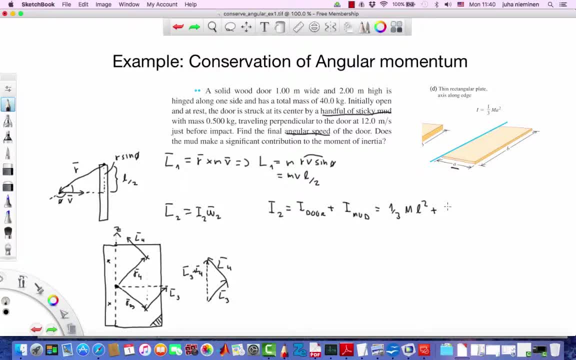 Moment of inertia is of course a mass or particle mass. so its moment of inertia is m times the distance, squared like this: And then we get L squared as a common term and we have m over 3 plus the smaller mass divided by 4.. 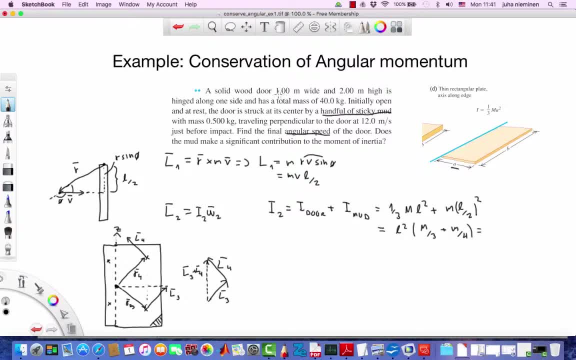 So the width of the door is 1 m squared. Door is 40 kg divided by 3, and the mud is half kilogram divided by 4. We get total 13.46 kg m squared and we see that the contribution of the, the mud, is pretty. 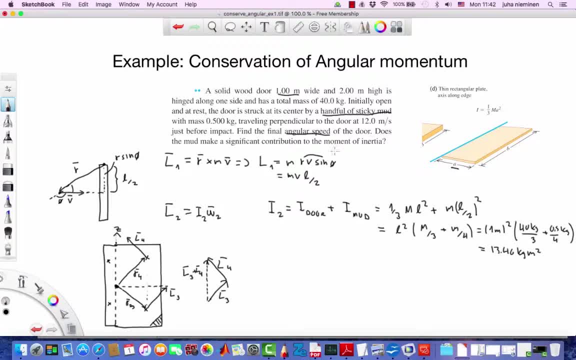 small because it's so light, and that was another question in this, in this problem. so does the mud make a significant contribution to moment of inertia? no, it doesn't, but we have it there anyway. and now momentum is concerned. so l1, the magnitude of l1, is same as magnitude of l2 and we get mv l. 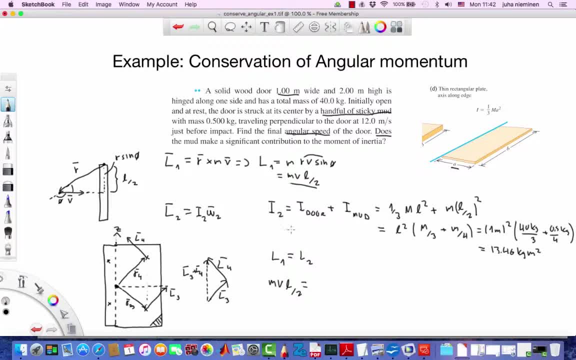 over 2 from here and from here we get for l2. so i2 times omega 2 and we can solve for omega. no, that is not a vector anymore. so omega after the impact that's going to be, and we L divided by 2 times i2, so the mass of the mud that's 0.5 kg. its velocity is